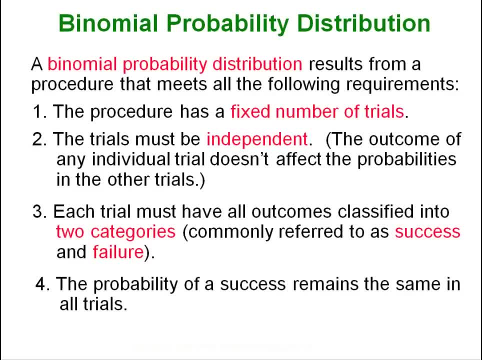 going to check Our previous results do not impact the probability of the next result happening. That's going to get a little tricky. let's say if you were picking a bunch of people out of a group, because as soon as you pick one person there's one. 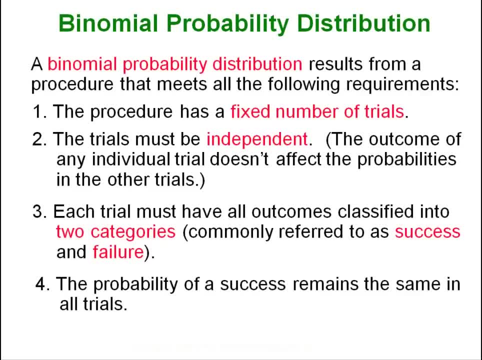 fewer person left in the group. so now the probabilities have shifted. But there are augmentations we can make to the procedure to make it seem independent. Each trial must have all the probability of the next impulse being triggered or the probability of it taking the same direction. Each trial must have all the probability of the next impulse being 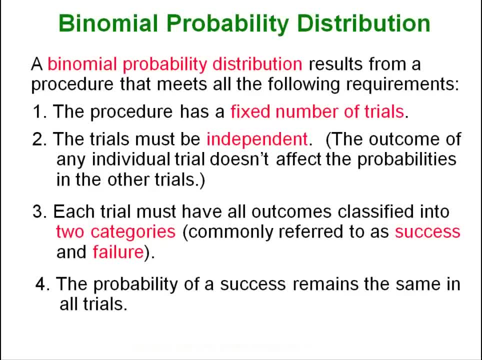 all outcomes classified into either successes or failures- Your two categories. So every time you run the experiment, the result you get has to go into one of those two categories. But as I said with my previous example, it's very easy to force a multiple category situation. 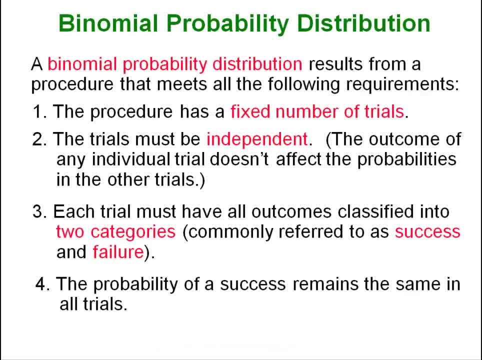 into two categories where you can just call them success and failure and you just define what a success is and it can be. multiple different outcomes can be considered a success and multiple different outcomes could be considered a failure. So you could group them into two different groups. And then the key here- and this goes back to kind of the independence. 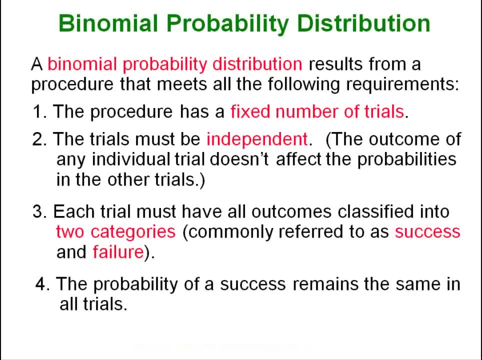 part as well is that the probability of a success has to be the same from each trial to the next, In its simplest case, every time you flip that coin. if a success means getting tails, that probability has to remain constant throughout the trials. Well, of course it. 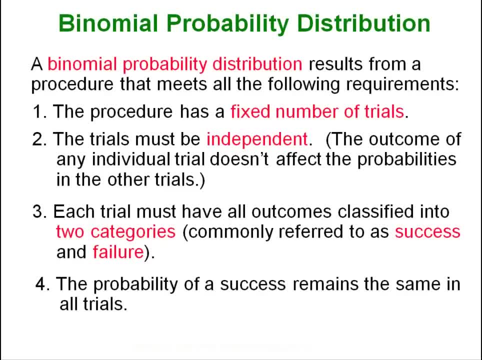 will, because the coin is not going to change. But you get the idea: if we were doing something else where we were picking somebody out of a group and they had to be a smoker and being a smoker was considered a success, then every time we picked that person out of that group, the probability that that person was a smoker 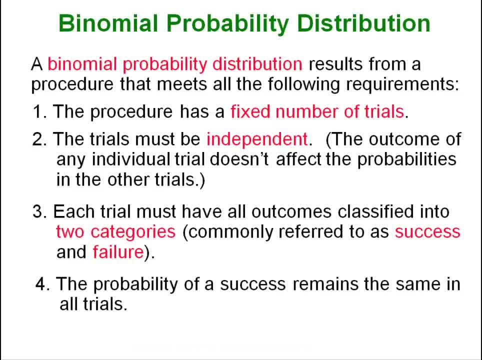 would have to remain constant, And that's going to be difficult when you are taking somebody out of a group and then not putting them back, because now the total number of smokers has changed, The total number of people has changed and therefore the probability has changed. 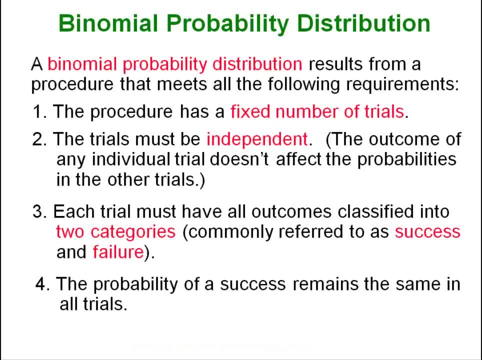 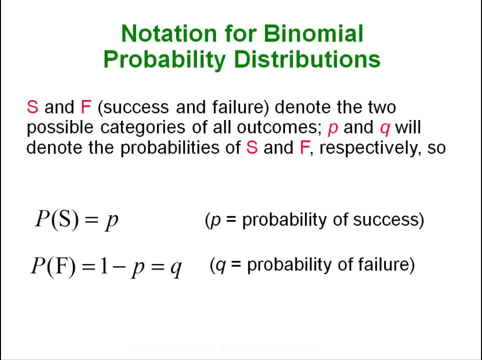 But, as I said, there are ways to kind of fudge the numbers if you need to. But with technology we don't need to do that. We would just use a different technique. Some of our vocabulary We are going to use success and failure instead of good or bad. 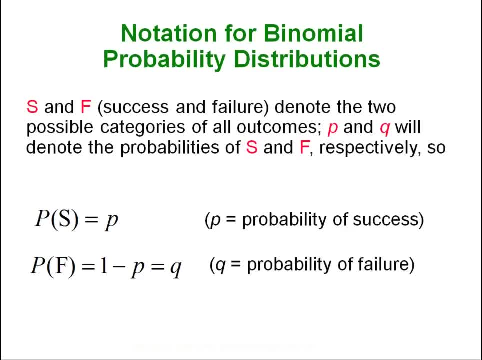 or yes or no, It's just the more commonly used terms for your two binomial groups. So when you see P of S, that's the probability of a success and P of F is your probability of a failure. And, of course, since these are two dichotomous groups and they make up, 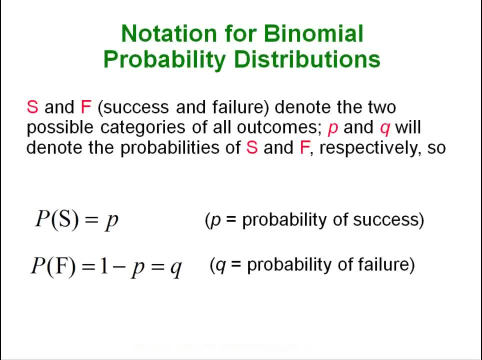 the entire sample space. their probabilities have to sum to one, So they are complements of each other. One minus P is going to equal Q, which is going to be the probability of your failure. So we are going to use P's and Q's: P for probability of success and Q for 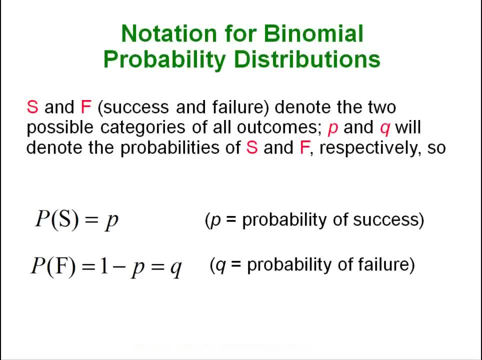 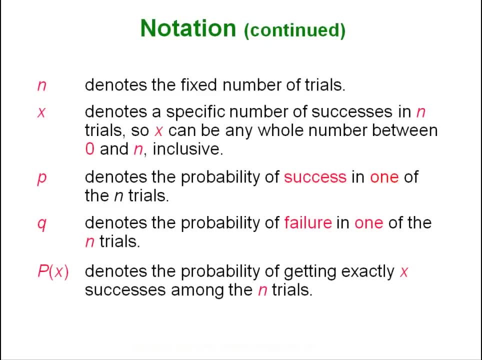 probability of a failure. No, this is not where, mind, your P's and Q's comes from, but it is another example of P's and Q's. Just like before, N is going to be the number of things. only here it's going to be the number. 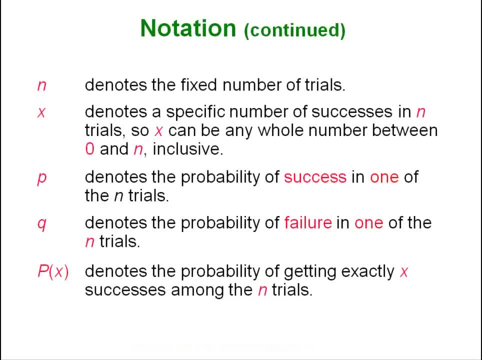 of trials. X is going to be the number of trials. X is going to be the number of trials. X is going to be the specific number of successes in your trials. So remember, it is coming back to that X that we had in the probability distribution. So X is going to be the number of good results. 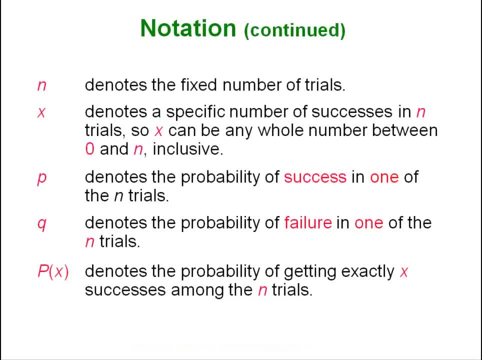 P is going to be the probability of a success in one trial, Not however many you are doing, but it is the probability of getting a success every single time you run the experiment. Q is the probability of a failure in one trial of the experiment. We know that P plus Q is 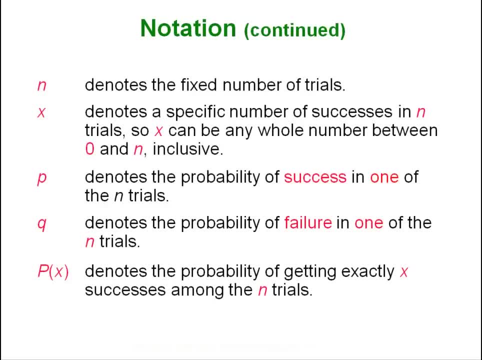 always going to equal P, Then capital P of X is going to be the probability of getting exactly X. many successes from however many times. If it was something as simple as flip a coin ten times, what is the probability of getting exactly three tails? then it would be P of three. Obviously, getting a tail was. 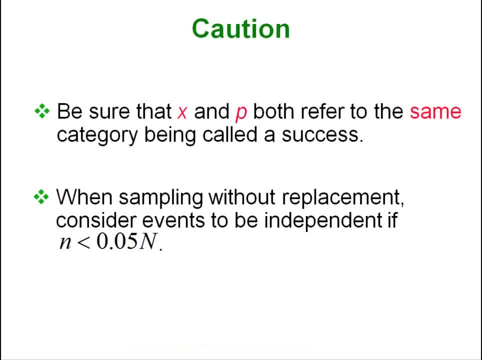 a success. Be sure, when you are setting up your trials and setting up your experiment you have to make sure that X and P both refer to the same category. So X is always the number of successes and P is always the probability of the successes. 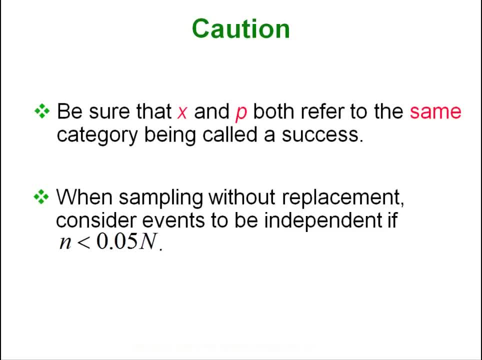 Sometimes it is not as clear as it sounds, because a success isn't a successful thing. Maybe you are trying to figure out whether or not using cell phones causes cancer, So you are looking back through a bunch of patient records and looking for patients who have. 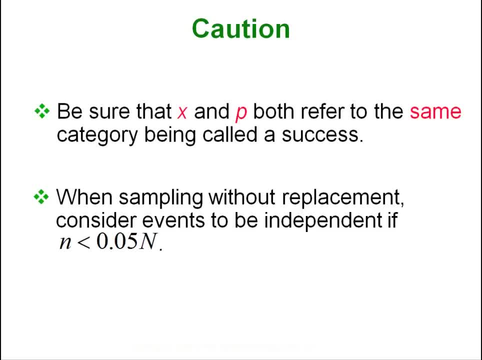 some form of cancer. Well then, finding a patient with cancer is considered a success, even though nobody would consider having cancer as being a success. So your X would be number of patients with cancer, P would be the probability of having cancer, and you would just need to make sure. 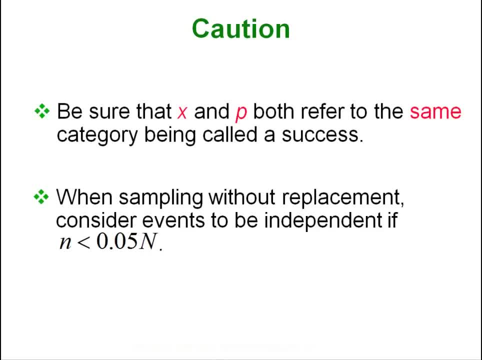 that, even though neither of those things are great, they are going to be considered your success case. Now, this was the thing I was talking about: forcing independence on something that really isn't truly independent If, when you are sampling without replacement, so you take somebody out of the group and 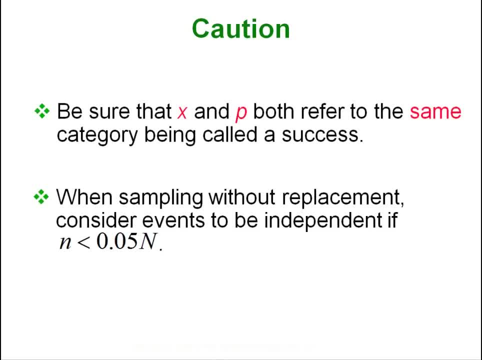 then you take somebody else out of the group and when you are doing that, the probabilities are changing every single time because you have less things in the group. I keep saying people, but it could be any kind of objects If you are going to, let's say, take a thousand. 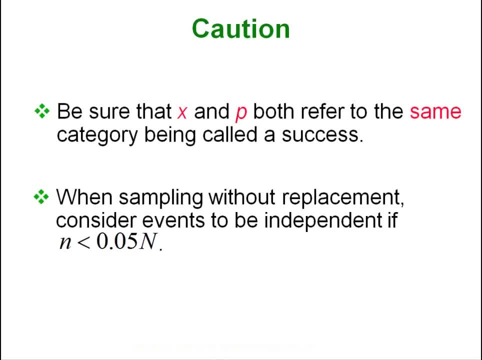 sample of objects from a big population. N, remember, is your sample size and then capital N is your population size. Right, Right, N is your population. So if the sample that you are pulling is less than 5% of your total population, then you can assume right. you can kind of fudge the numbers and let the 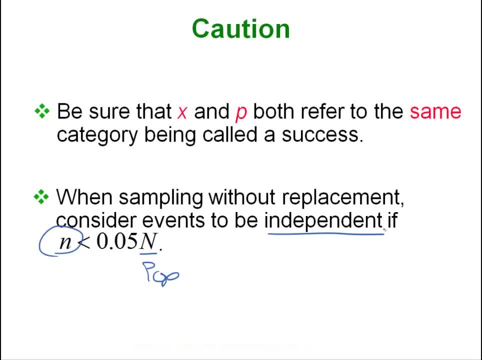 trials be independent. Even though we know they aren't going to be independent, the difference from one to the next is going to be so small, because the sample is so small relative to the entire population, that that slight change in probability you can go ahead and just ignore. 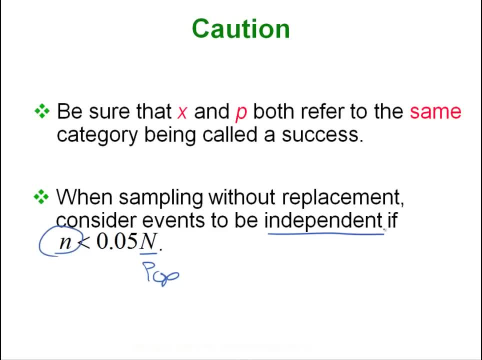 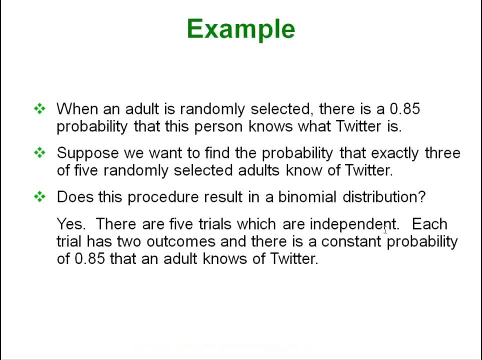 it and let it all be independent. As I said, we also have stronger technologies to deal with these types of cases, where we no longer have to do these kind of fudging of the numbers. Here is a good example. So we are going to randomly select an adult from amongst all adults. So just go out there and 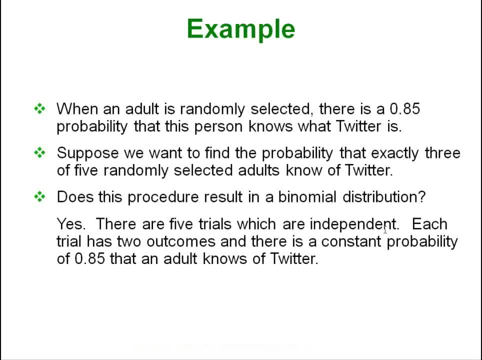 choose someone on the street. We know from previous, let's say- surveys and things like that that 85% of the population knows what Twitter is. So that means that if we just chose an adult at random, there is an 85% probability that that person knows what Twitter is. So 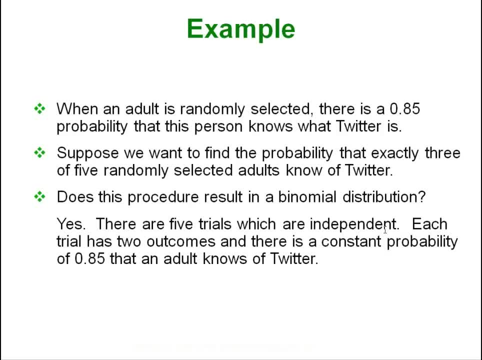 suppose we want to know what is the probability that if we went out and chose five people at random, exactly three of them would know what Twitter is. You are kind of asking who the hell cares. That's kind of a stupid question. Yes, it is, but this is just a learning tool. 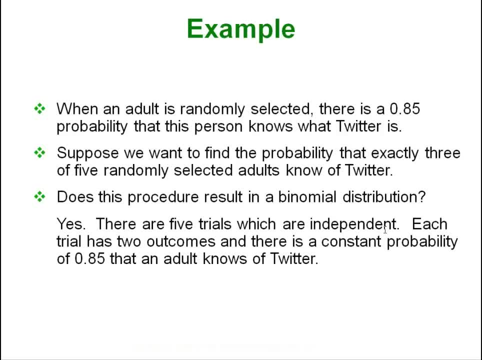 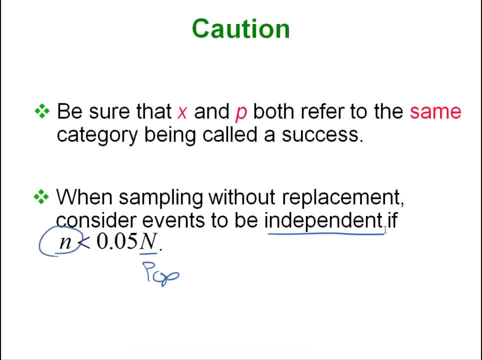 But you get the idea. So we are going to pick five people at random. We want to know what is the probability that exactly three of them know what Twitter is. Is this a binomial distribution? And yes, if you go back and look at the rules, right? is there a fixed number of trials? 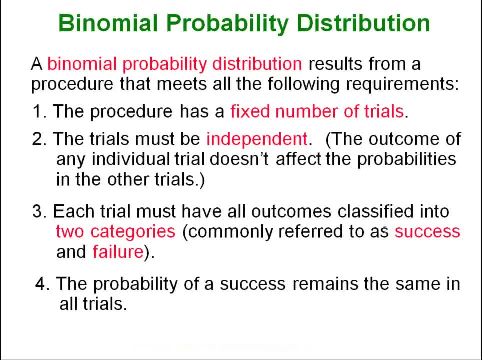 Yes, And in this case, what is our number of trials? And hopefully you are all saying five, because we are picking five people. The number of trials is not three. Three is how many successes we are looking for. That's going to be our x. The trials must be independent. 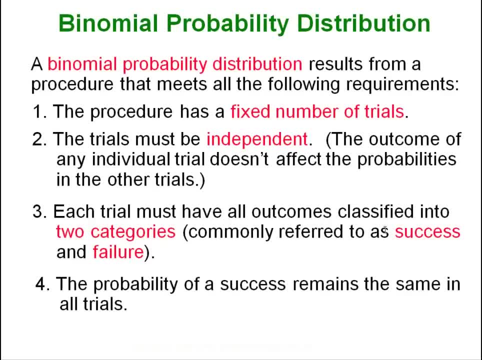 So that means picking one person shouldn't have any influence on the other person as far as changing their probability. And, yes, they are totally independent. Each trial must have outcomes classified into two categories. Well, either they know what Twitter is or they don't know what Twitter is Right. So either it is a success or a failure, So that's. 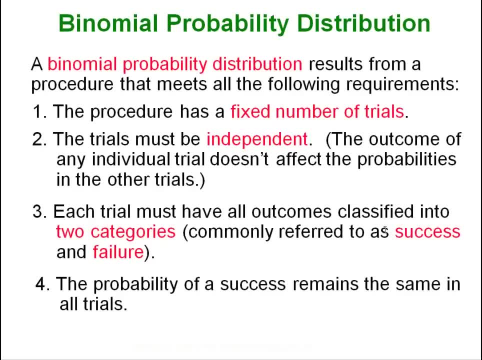 true, And the probability of a success has to be the same in all trials. And since we know 85% of the entire population knows what Twitter is, then doesn't that mean every single person has the same probability of knowing what? there is an 85% chance that this person 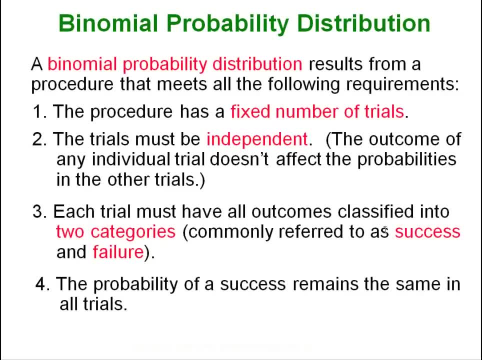 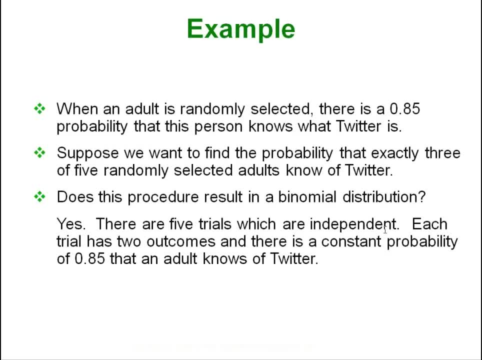 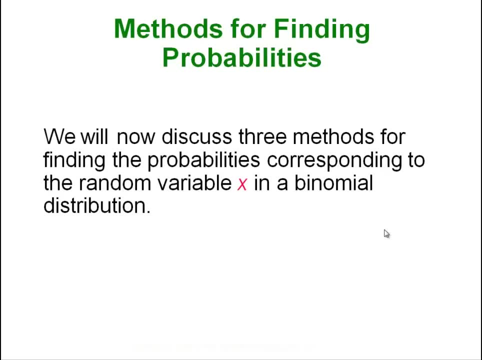 knows it and there is an 85% chance that that person knows it. So the probability remains constant. So it fits all the key criteria and therefore it is yes. in fact it is a probability distribution. Methods for finding the probabilities: there are three ways, Really. 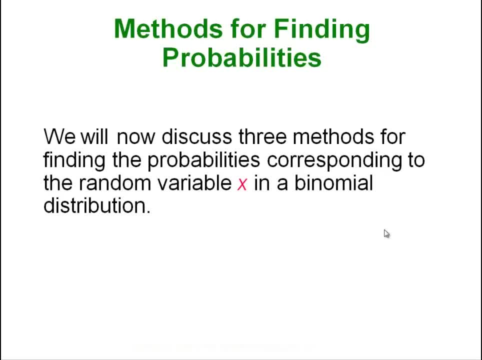 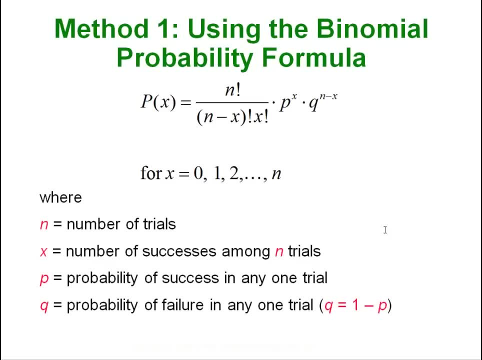 three ways. just to think about it, There is really only going to be one way we are going to use it, and that's going to be technology. So the first way is to use the formula, And I want you guys to take a second and look at this formula, because it does help you understand. 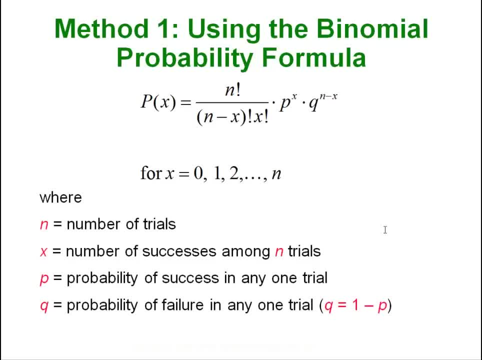 what a probability distribution really does. So let's kind of go back to the previous example of picking five people And we want to know the probability that three of them know what Twitter is. So here's my five dashes: One, two, three, four, five, Right, And exactly three of them have to know. 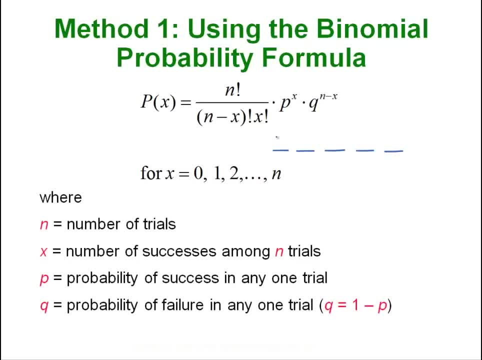 what Twitter is. So let's let the first three people know what it is. So it's going to be .85.. Right, .85 and .85, because that's the probability that a person knows what Twitter is. But if these last two people don't know what Twitter is, what would the probability? 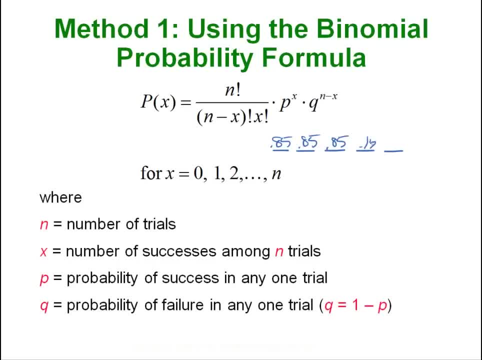 of choosing them be. And yes, it is the opposite, Right, The complement of one minus that, So .15. The 15% chance. Now look what we get If we multiply these together, because this is to figure out the. 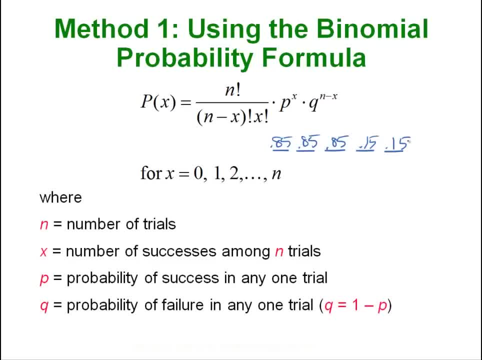 probability that this happens. we always have to multiply our dashes. So if you multiply all those together, that's going to give you a number that represents three who know what Twitter is and two who don't know what Twitter is. And if you look at this formula up here, 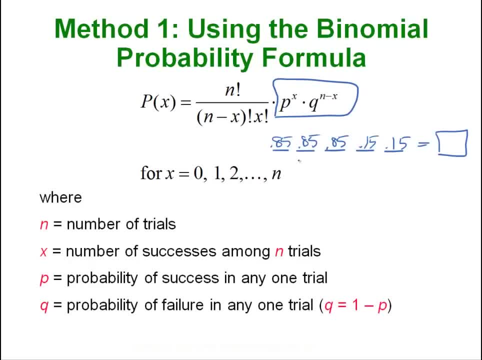 it ends up giving us this piece of the formula, Because the probability of knowing Twitter our p, the probability of a success, was .85 in this case, And the probability of a failure was .15.. So this ends up being p, p, p, q. 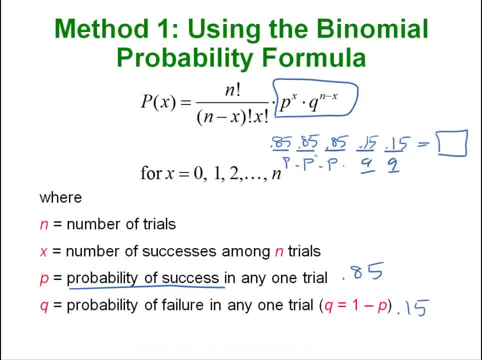 and q And if you multiply three p's together that's p cubed Right, Where x is the number of successes. In this case we wanted three successes out of five tries. So you can see how these numbers give us that part of the formula. So this end part of the 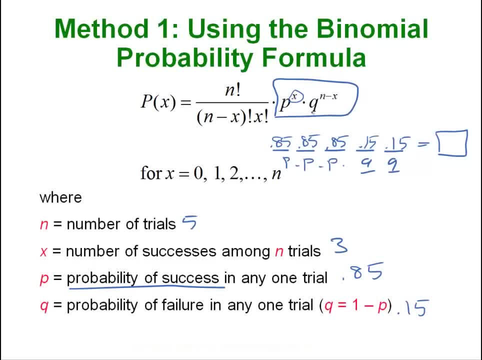 formula is just multiplying together the probabilities of those successes and failures. If we have three successes, then we end up getting .85 cubed times the probability of failure raised to the power of the number of failures we have, which in this case is 5 minus 3. Right. 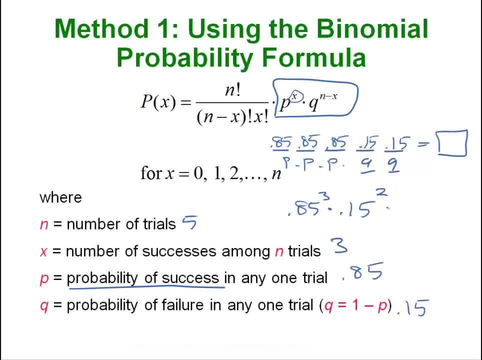 5 minus 3 and minus x, Which is two of them, And that's the exact same thing we got with our dash technique. Now, what about this? What's all this junk? Where does this come from? Hopefully you recognize that as one of our factorial formulas that we learned in our section on probability. 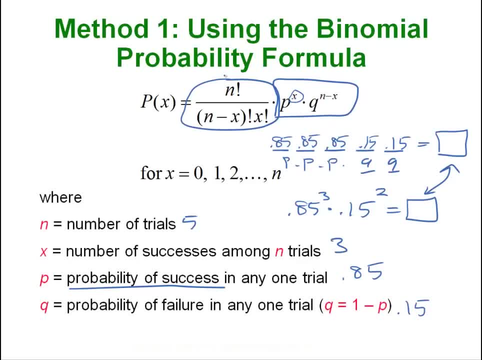 And which factorial is that? Is that a permutation or a combination? If you don't remember, pause the video and go look back through your notes, or you can wait a second and I'll reveal all. It is, in fact, a combination. That is, the combination of n choose x, Right? I know we normally used n's and r's when we 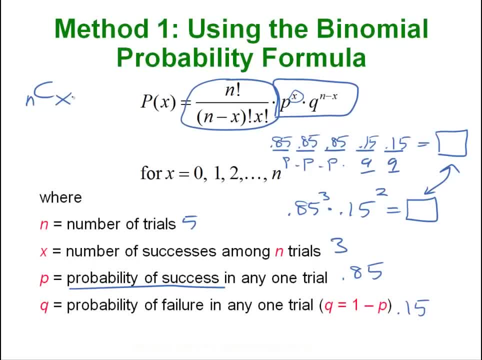 did the formulas, But it's the same thing, Right? So we have n many things and we're going to choose x many of them. This formula tells us how many ways we can take these three p's, these three successes, and these two q's, these two failures, and rearrange them. 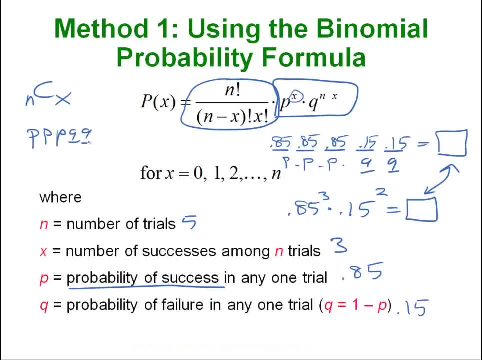 So it's counting up P, p, p, q, q, but it's also counting up p, q, p, p, q, et cetera, et cetera, et cetera, All the different ways you can rearrange those p's and q's. that's what this combination does. 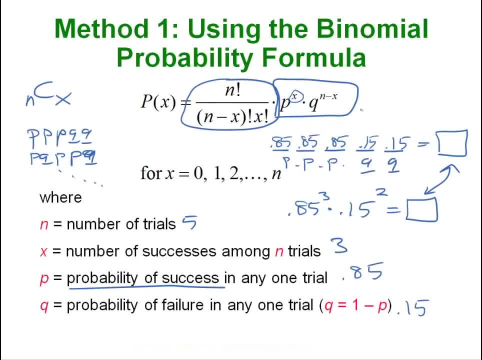 It counts up all those ways. Well, if I rearrange the .85's and the .15's, put them in a different order, when I multiply them together, won't I still get this exact same number? Won't I still get the same number that's going to be in that square, whatever that happens to? 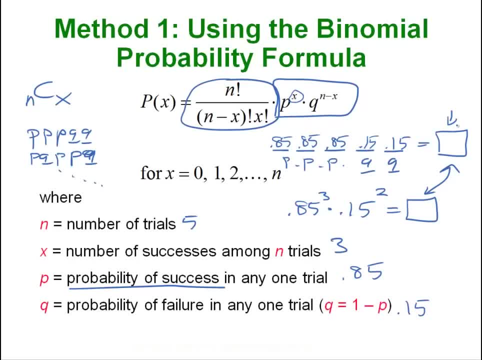 be? Because we all know that A, A times b is the same thing as b times a. So if I rearrange all those numbers, I'm still going to get that same number. So if it turns out that I can actually rearrange them ten times, then aren't I just going to? 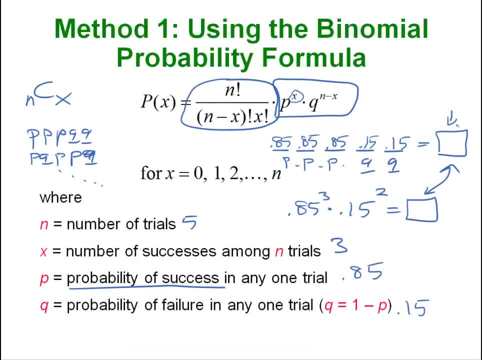 get ten of those numbers. Let's say that number was .2.. I'd get ten of them. I would add them all together and that would be my probability, which would be a problem because it would be bigger than one. So obviously it's not going to be that, but you get the idea. 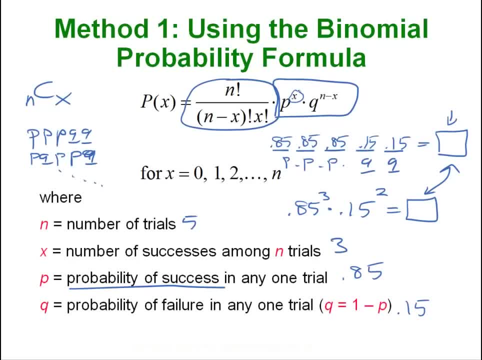 So this formula just says that, hey, This is. Let's see, This is the probability of x number of successes and the rest being failures. This is the number of ways that you could rearrange them. get them in a different order, Right? 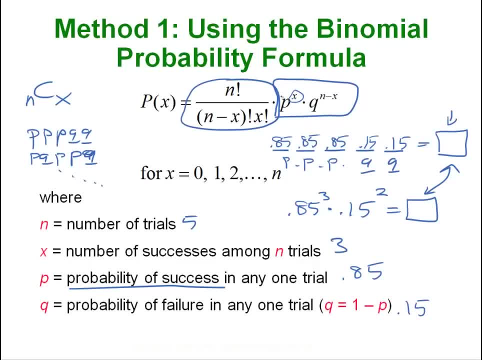 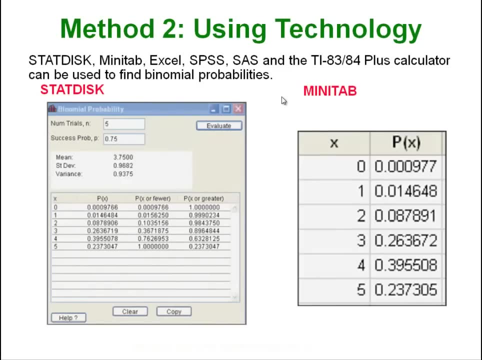 And when you multiply those two together, that gives you the total of all the probabilities of all those different arrangements, and that's the binomial probability formula. It's very simple. Don't worry about memorizing it, because method two is using technology, Whether you want to use stat disk or stat crunch or mini tab or your calculators or 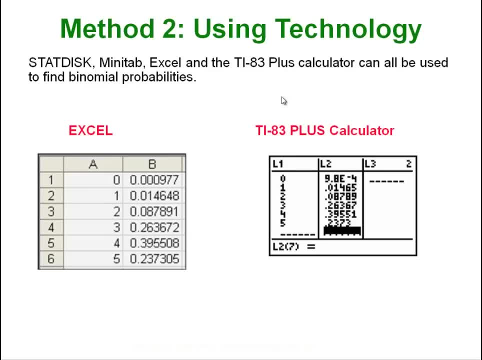 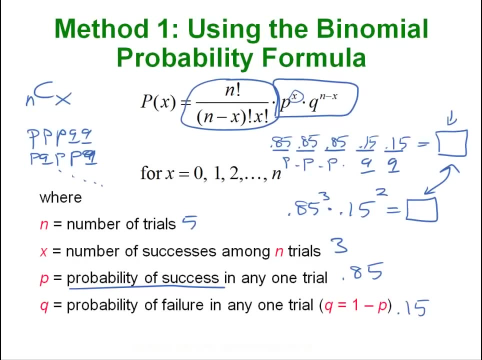 excel, all of these things will run binomial probabilities for you very easily, So there's no need to memorize that formula and use that formula. I like to look at the formula because it kind of helps us understand what's going on with the binomial formula. 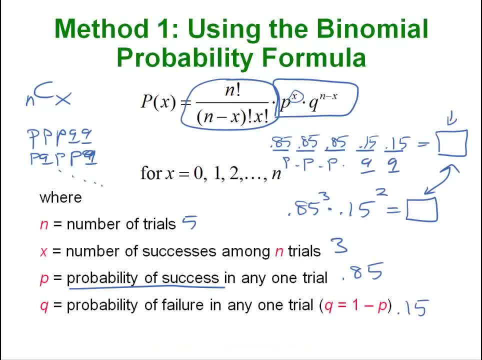 What's it doing? Why is it doing what it's doing? It gives you a better idea. It gives you a better understanding of what binomial probability really is. It's just telling you the likelihood of getting x number of successes out of n number trials. 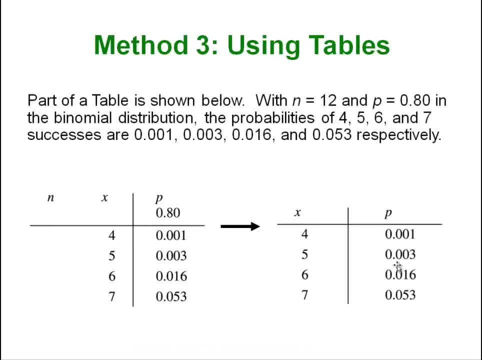 So in this case, three out of five people know something. Method three: using tables. don't even want to waste time with it. That would be almost worst case scenario. Tables are very limited. You have to have the right number of x's and the right number of n's, and they are very 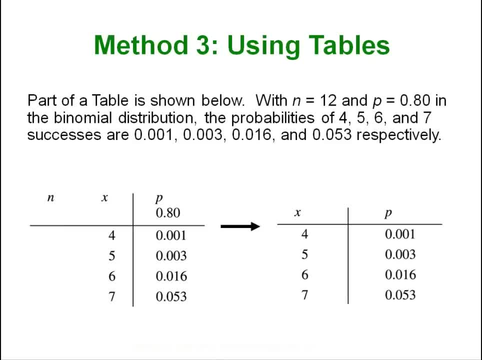 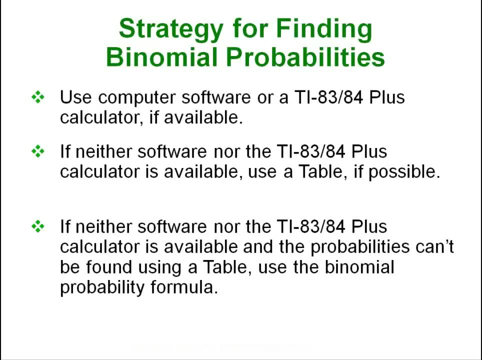 very limited. It's only something you would use under very, very small circumstances. Obviously, the first thing we always want to do is try to use technology. If we don't have technology, a table would be easier under certain situations, But if the numbers don't allow it, then we have to fall back on using the formula. 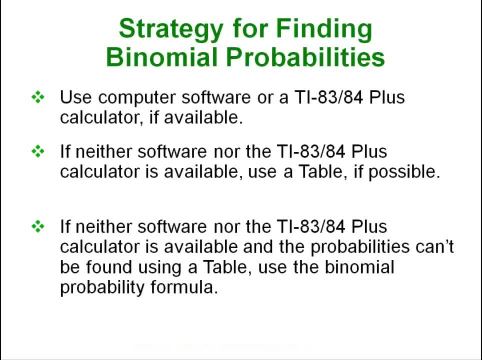 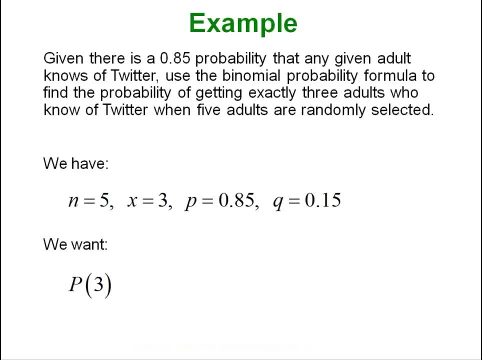 But unless there is a global blackout, why would we not have technology? Here is our example that we worked out before: Right, The x's and the n's, Three successes out of five. Probability of a success is .85.. Probability of a failure is .15.. 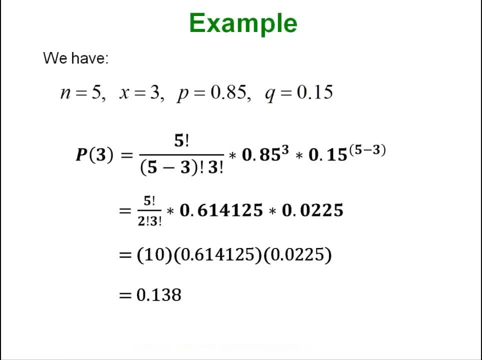 So we are looking for p of three, We are looking for three successes. Here is everything thrown into the formula: N is five, X is three. Right, Our success rate is .85.. Our failure rate is .15.. Put in the three. 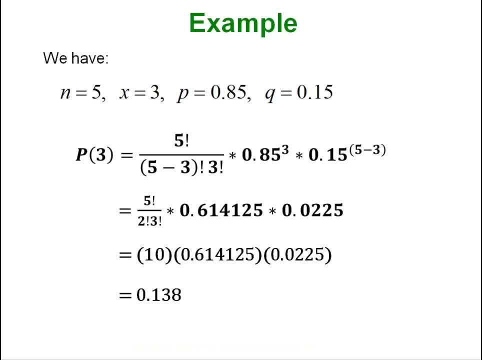 Put in the five minus three, Calculate all that stuff out and it ends up being .138, or almost 14%. And it's not that bad And it's as simple as that. Again, technology will do it for us. lickety split, We've gone through this. 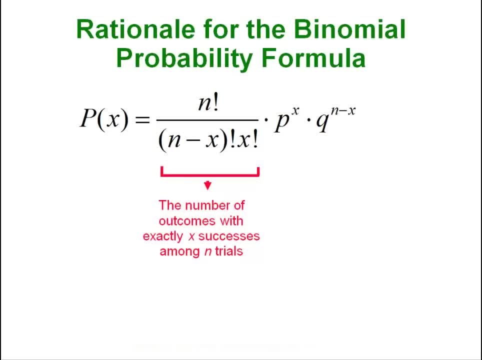 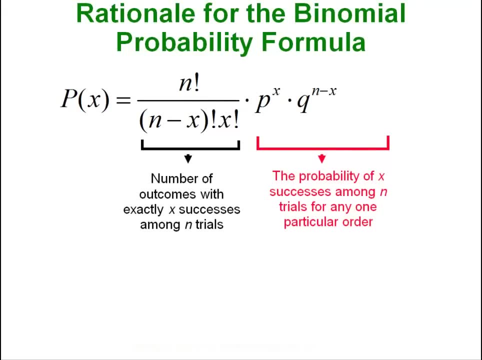 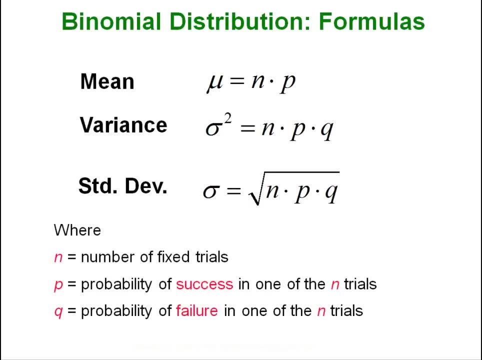 That first number shows us the number of ways we can rearrange our p's and q's. The second part gives us that probability of that arrangement of p's and q's and when you put it all together it gives us the total probability. Just like any other probability distribution, we can calculate means and standard deviations. 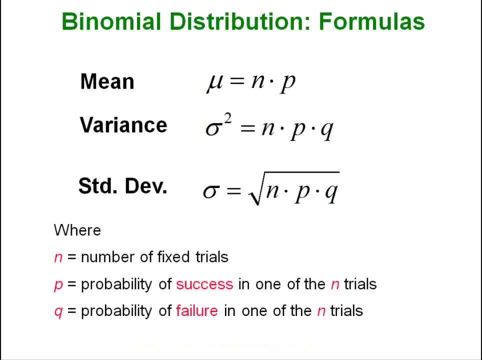 What is the other word for mean that we use sometimes? That is right: Expected value. You will also notice that these formulas are extremely simple, Right? I mean? how could it get any easier than just n times p and then npq, square root for standard. 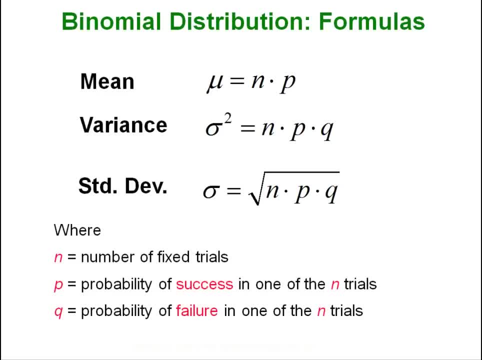 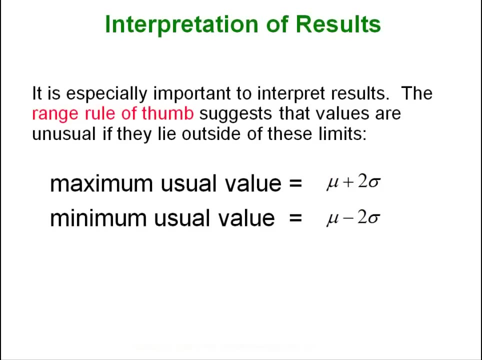 deviation. So those are two of the easiest formulas you are going to see in this entire, in your entire statistics career. So those might be two that you might want to memorize, but then again, who cares? throwing it into technology, Technology will do these for you as well. 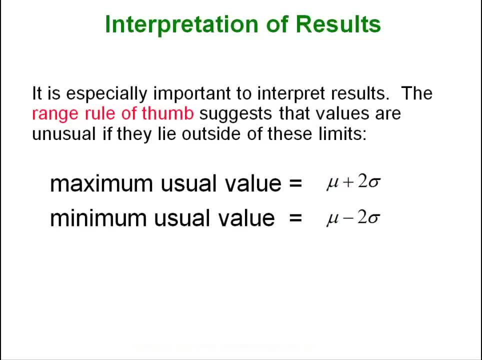 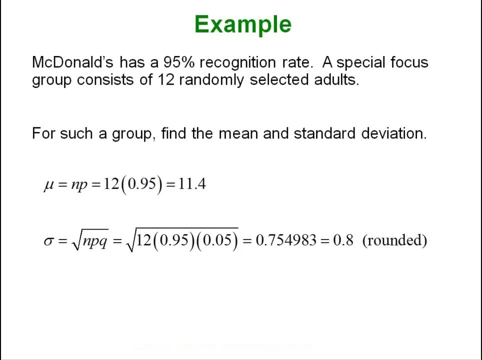 Just like before, we have the range rule of thumb, The unusual and unusual stuff, and just like before, it's always your mean plus and minus, two standard deviations. Here is an example: 95% of the world's population recognizes McDonald's, and that's actually pretty accurate. 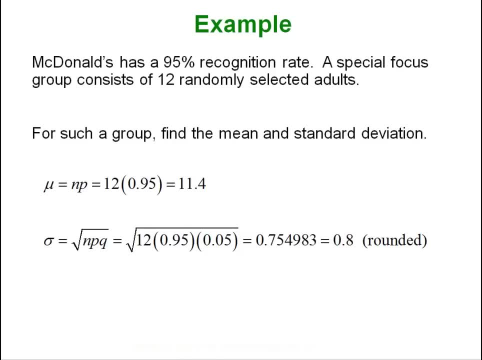 If you went out and just randomly chose McDonald's, That's actually pretty accurate. If we chose a focus group of 12 adults, we could find the mean and standard deviation of the number of people in that group who recognize McDonald's. So in this case our sample size is 12 and our p is .95, because that's the probability. 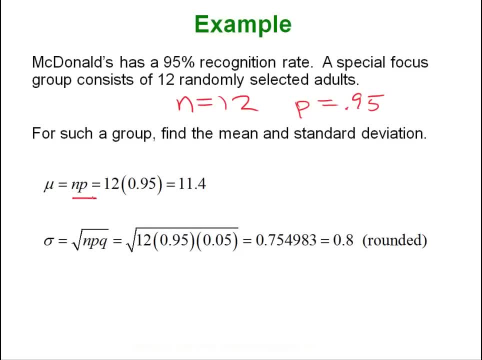 of a success. So the mean right is just n times p, And we would expect that out of a group of 12., 11.4 of them would recognize McDonald's. Now you're probably asking: how the heck do I get a .4 of a person? 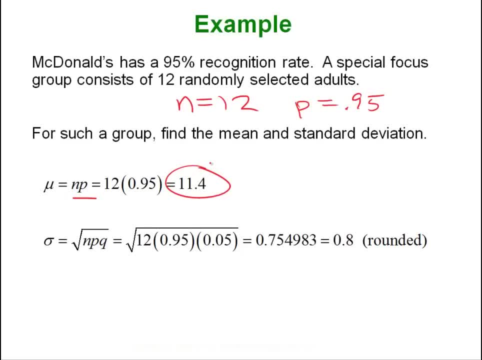 You don't, And that's something to realize: that an expected value doesn't always make sense in the real world. You can't have 11.4 people out of 12.. But what the expected value means is that, on average, if you randomly chose 12 people, 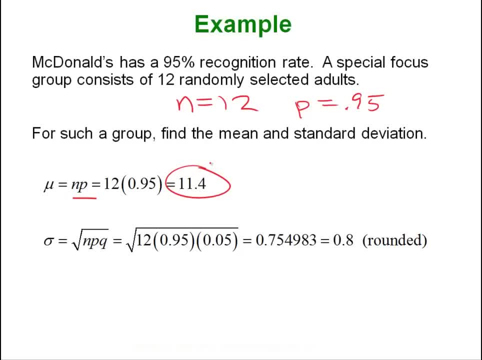 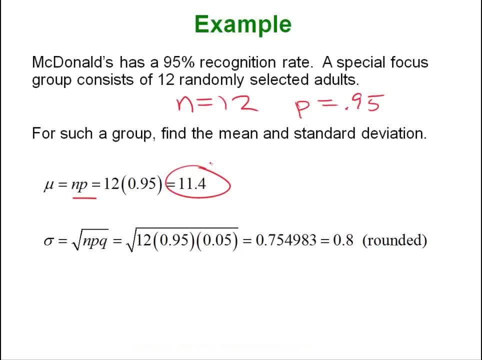 Now, really, the message is that if you actually ran that experiment over and over and over and again and each time wrote down the number of people from that sample that recognized McDonald's and then took the average of those results, you took the 12's, the 11's, the 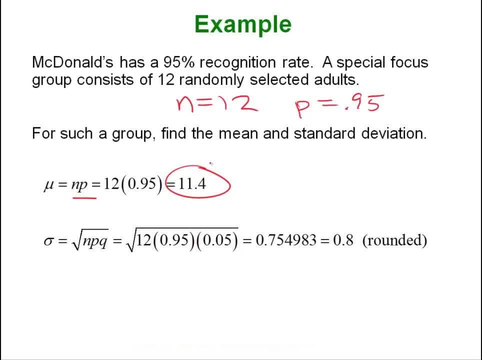 10's that came up here now, and then maybe you even had a group that only 9 recognized it. you add all of those numbers together, divide by how many times you ran the experiment, then you would get an 11.4.. That's what the expected value means. is that, on average, if we ran this experiment over 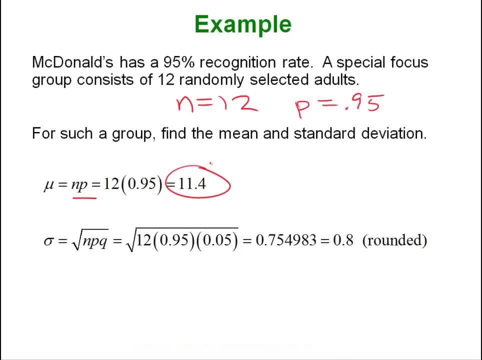 and over and over again. we would expect 11.4.. As the average number of them, Germany as the average number of people who recognize McDonald's. Okay, And then the standard deviation of .8 when we round just tells us how spread out those numbers are, and it also can give. 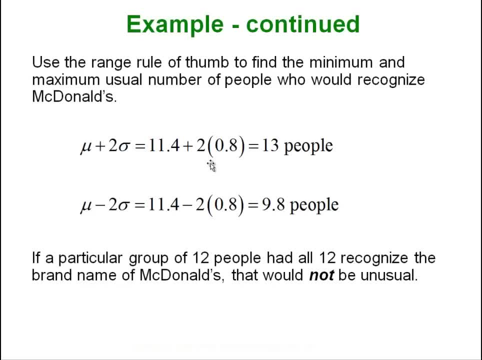 us an idea of unusual results, which is what we do here. We take that .8 and multiply it by 2. We add it and subtract it from the mean and we can see that, on any given random selection of 12 adults, if we had 13 or more people recognizing McDonald's, it would be considered unusual. 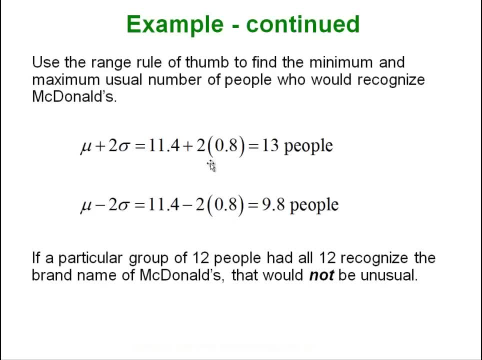 and you go: no duh, because we only grabbed 12. so how can we have 13 or more? Again, silly result, only because the numbers are so small. But on the other end, if we had 9.8 or fewer, that would be considered unusual. So 10 wouldn't be considered unusual, but 9 would. So if we 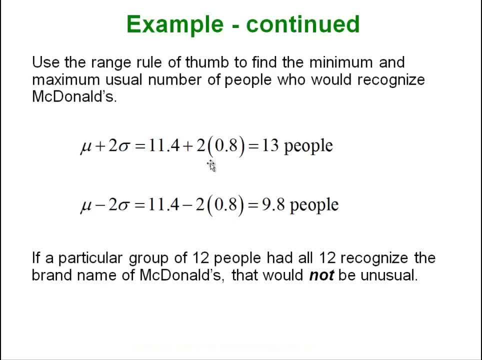 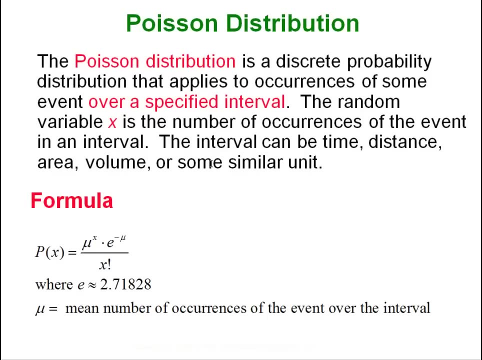 got a sample of 12 and only 9 of them recognized McDonald's. that would be considered unusual, An unusual result, And that's the end of binomial distributions. Now there is a related distribution called Poisson distribution, And you can probably stop the video here if you are not going to. 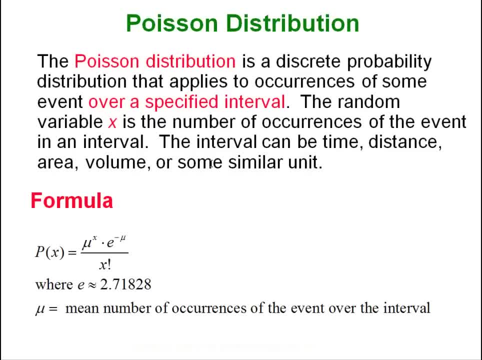 do Poisson distributions in your class, But if you want to learn about a slightly different distribution, this one comes up a lot in the real world. It is actually a pretty important distribution, So hopefully you are going to cover it in your class. It's still a distribution. 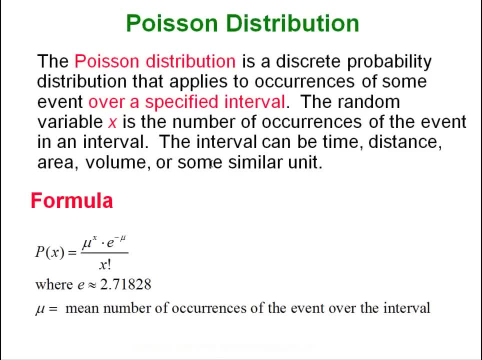 Discrete probability distribution, just like binomials. The only difference is we use this distribution when we are looking at occurrences of some sort of event or experiment that happen over a specified time interval. So the random variable x is still the number of successes right or the number of occurrences of the event, But instead of it just being the number, 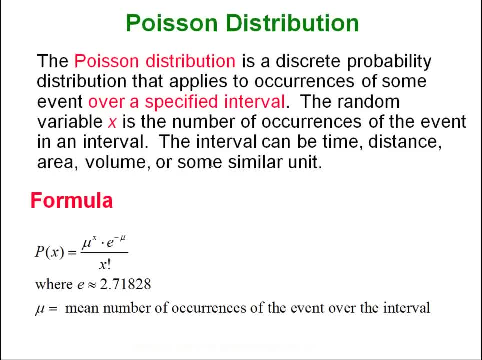 of successes out of n number of trials- right, so we are not going to say we are going to pick five people, It's probably three of them know something. It's the number of successes that we get over a time interval or some sort of interval, Usually time, It can be distance, area, volume. 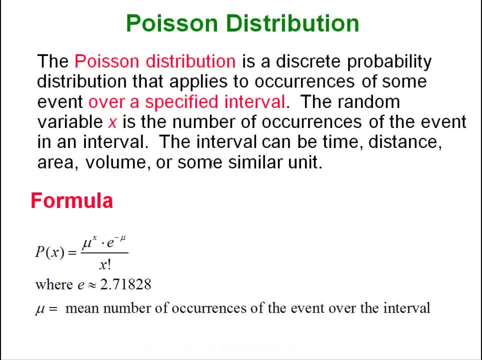 or some other measurement, But time seems to be the most widely used version of this, So you can see how this would have a totally different application. It's no longer pick 12 people and find out how many of them understand or recognize McDonald's. It would be sit at. 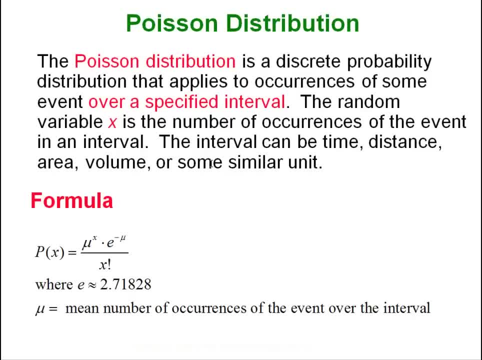 an intersection. It would be: sit at a car and watch cars go by and in a one hour time period, how many of those cars are hybrids or electric or some sort of alternative energy vehicle? That would be a very timely question. no pun intended, And we would need to do a Poisson distribution. 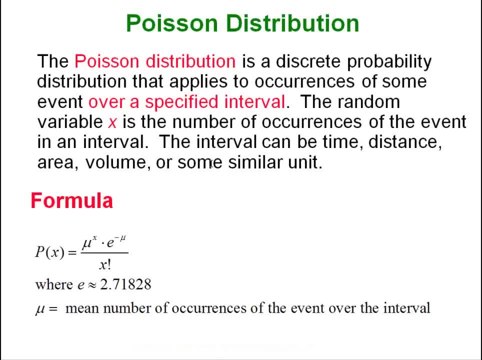 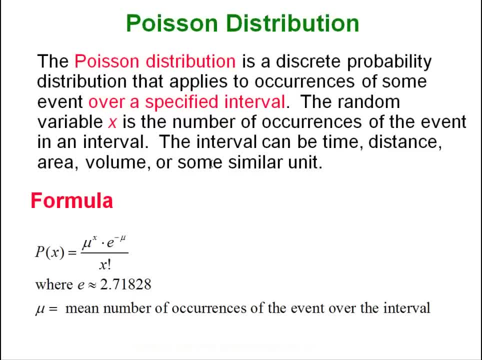 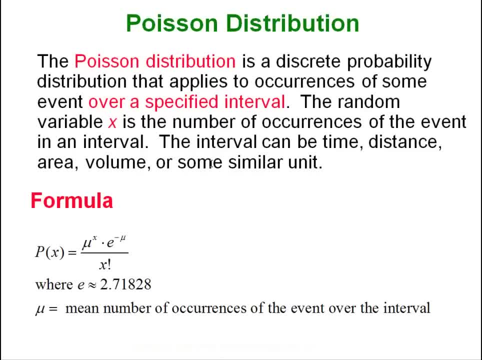 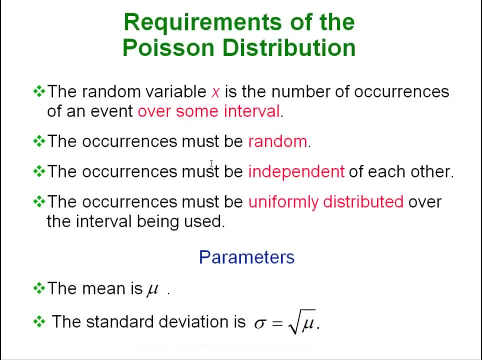 hopefully seen before. 2.71828: blah, blah, blah blah. Similar to pi, It's an irrational number. So they are pretty easy numbers to deal with and, just like before, technology will do it all for us. The requirements for this distribution: the random variable x is the number of occurrences. 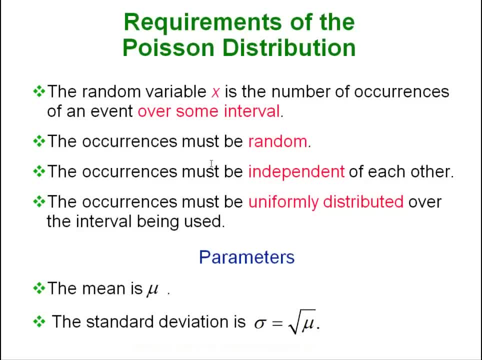 just like before, only now it's over some interval rather than out of a certain number of trials. occurrences need to be random and independent and they need to be uniformly distributed over the interval being used. So that means you can't have peaks and valleys, You can't. 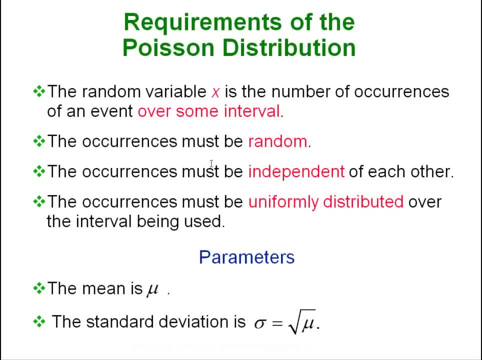 be more likely to see hybrid vehicles in the first five minutes of the hour than the last five minutes of the hour. or if you were going to do it over a week, you couldn't do this if it was more likely to see hybrid vehicles on the weekend versus during the week. So 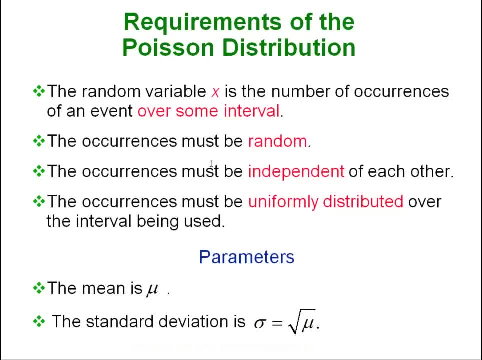 it needs to be uniformly distributed. It should be equally likely that a hybrid vehicle would travel through that intersection at any given point in time. for the example that we are talking about, The mean is very simply just mu and the standard deviation is really simply just the square root of mu. 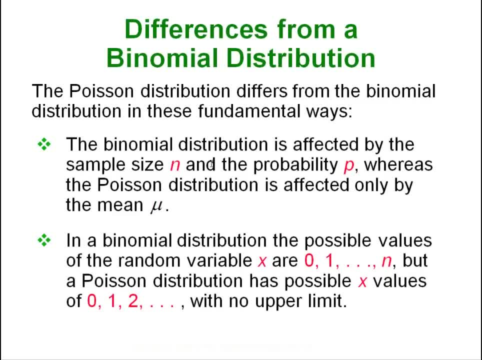 Big differences between the two. The binomial distribution is affected by a sample size and the probability, whereas the Poisson distribution is only affected by the mean. A binomial distribution has possible values from zero up to n, because you are only going to do n number of trials, so you either 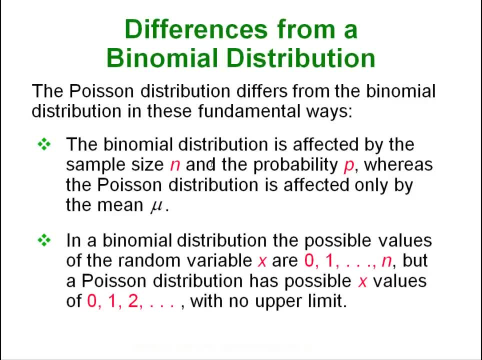 get no successes all the way up to all n of them. but a Poisson distribution has no upper limit. In that one hour no hybrid cars could go by or you could have a million go by. So there is theoretically no upper limit to x on a Poisson. 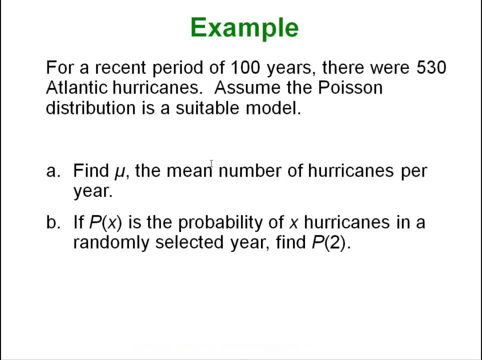 distribution. Here is a good example. So if we are looking over a period of 100 years, there were 530 Atlantic hurricanes. So we want to assume that the Poisson distribution is a suitable model. So that assumption means that hurricanes are evenly distributed over. 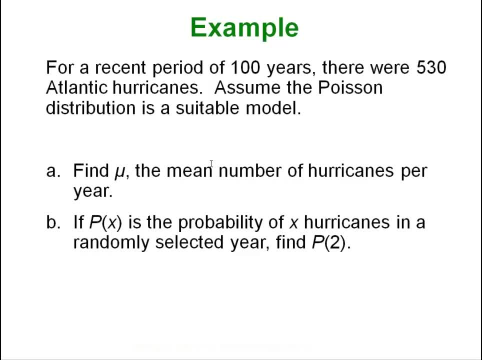 those 100 years Right? There shouldn't be a higher probability. There should be a higher probability of seeing hurricanes in one year to the next. We want to find mu, the mean number of hurricanes per year, and then if p of x is the probability of x hurricanes in a randomly 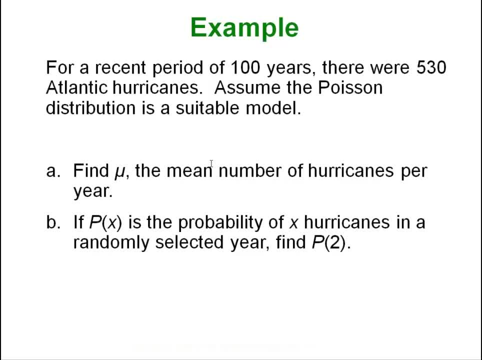 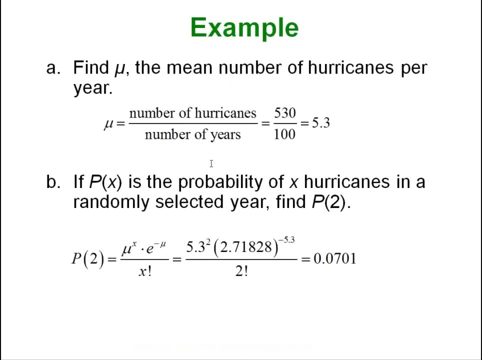 selected year. we want to find the probability that we have two hurricanes in a randomly selected year, which would kind of give us an idea of what is the probability that we have two hurricanes next year. So you can see how this could actually be a reasonable thing to do and kind of an important thing to do. 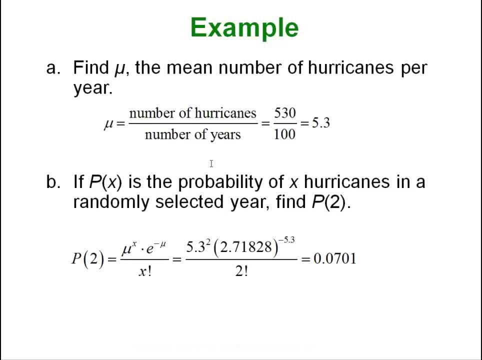 Here are the numbers. Very simply, mu is just the mean that you would expect Right Number of successes over total number of things. We had 530 hurricanes in the last 100 years. So 530 divided by 100 we had 5.3 hurricanes per year. That's the average. Now to figure out p of x, we very 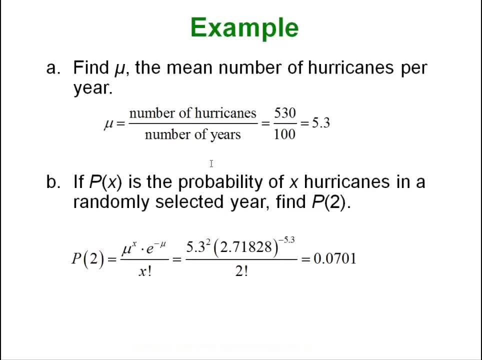 simply put those numbers in. So p of 2 is just mu, the 5.3 squared times e to the negative 5.3 over 2 factorial. You work it all out and it is 0.07.. So there is a 7% chance of. 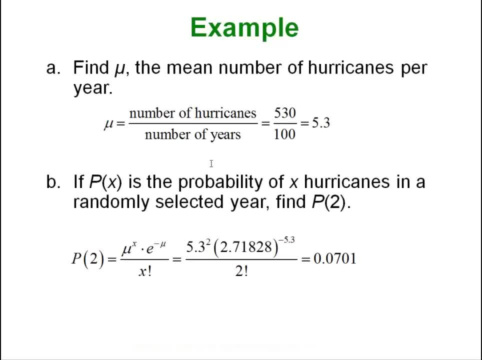 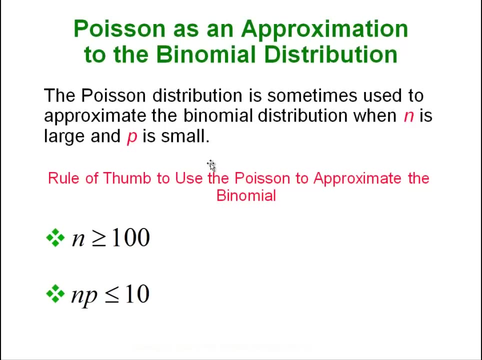 having exactly two hurricanes in one given year. You might think that is kind of small, But it is kind of small because this is the question of exactly two, not two or more. So that is a totally different question. You can use the Poisson to approximate the binomial. 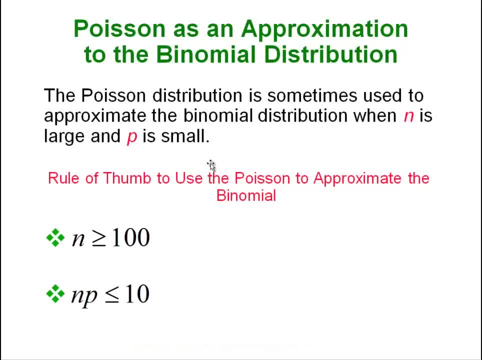 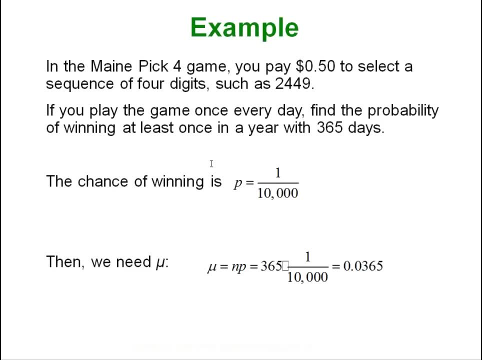 but why would you, Since we can already do the binomial process? Well, we can't do the binomial, so you can ignore this and ignore this and, in fact, ignore the rest of the slides. You can read through it and see how it used to be done, but this was really a technique. 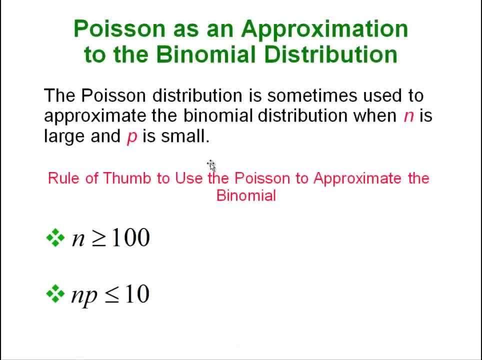 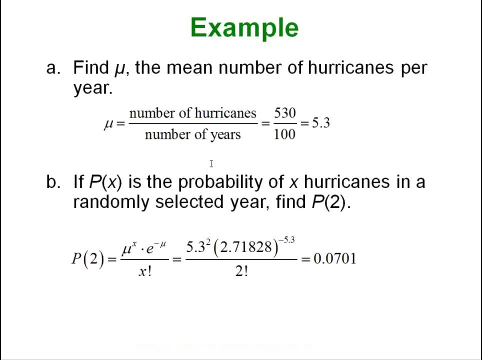 that was only needed before technology came around, because this was actually a little easier to calculate. but ignore it. We'll just stop with this nice example of the probability of 2 and remember that's too specific If you want to know the probability of 2 or more. 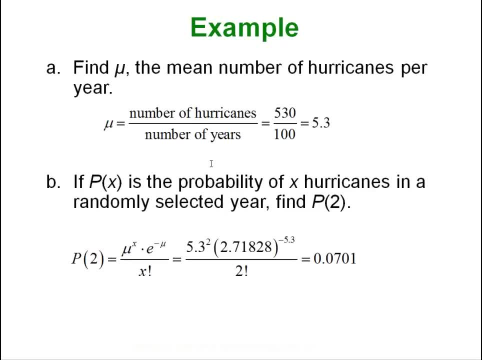 you would have to do something completely different, and then, of course, the probability would be a lot higher. That's it.